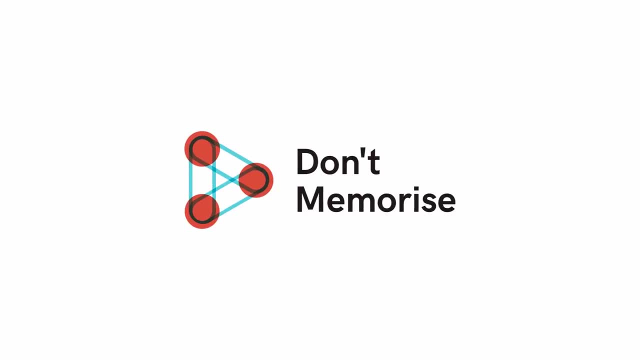 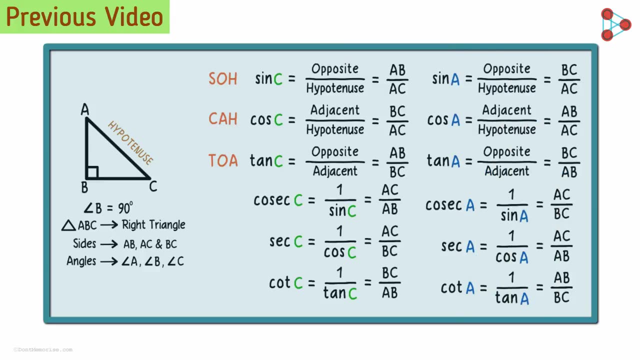 In the previous video we saw basics of trigonometry. In this video we will see some of the applications of trigonometry in real life. Trigonometry has lots of applications in the real world and can be used in many practical situations around us. 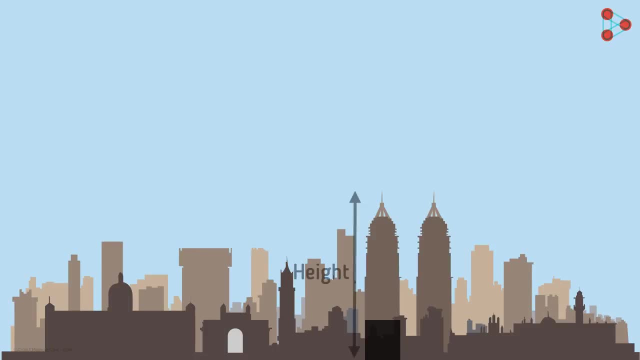 They are mostly used in finding the heights of things such as towers, buildings, or they are also used to find the distance between two things. How do we find these heights and distances using trigonometry? Let us see that with the help of an example. 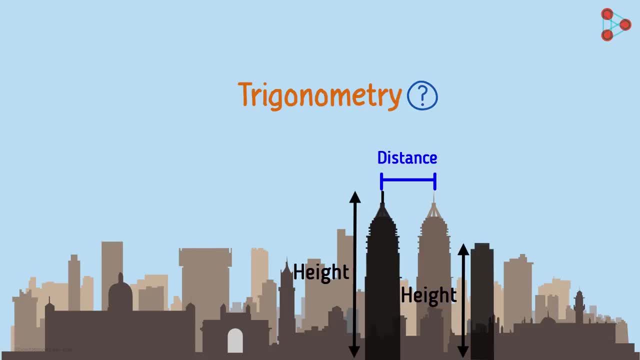 But first let's talk of one more important thing before I put a question. on the screen, We have seen trigonometric ratios of angles of a right angle triangle. Hence, forming the right triangle from the given question is the most important step while solving problems. 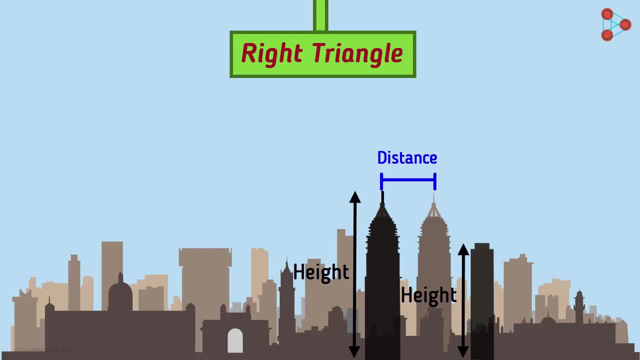 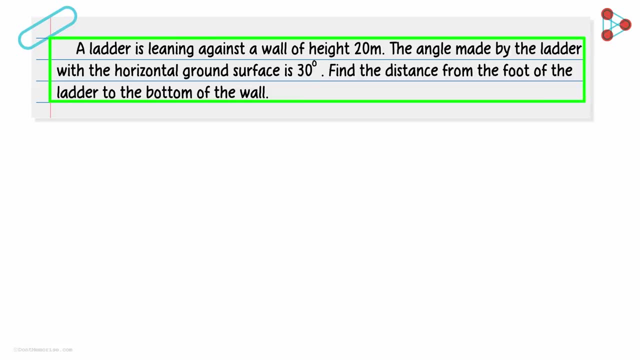 Now I will put a question on the screen And you try to sketch out a right triangle from the given information. Let's start with a simple example. Read the question carefully and try to form a right triangle. Here we are given a wall. 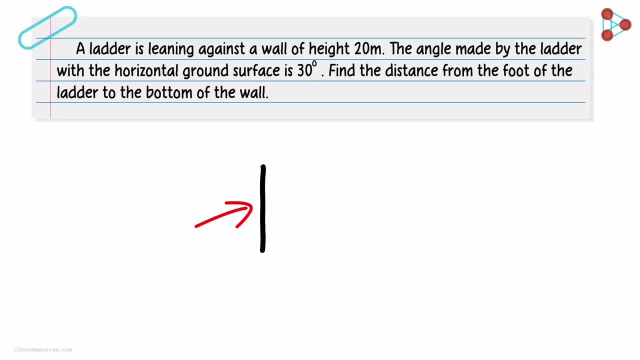 You can't represent the wall with a vertical line like we have done here? You don't really need to draw an actual wall Now. it's obvious that this wall makes an angle of 90 degrees with the ground surface. So you can draw a vertical line like we have done here. 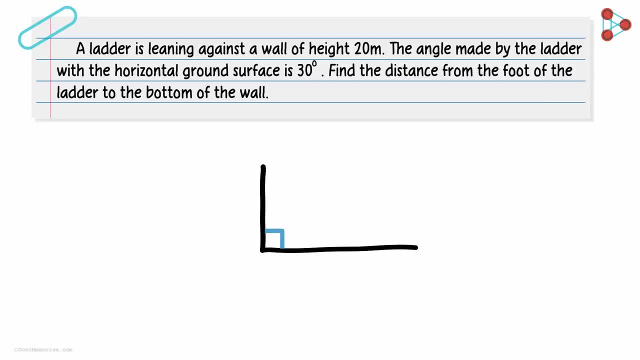 And finally, we are asked to find the angle with the ground surface. That's something we can definitely assume. We are also given the height of the wall. as 20 meters, A ladder is inclined against the wall like this. Again, you can represent the ladder with the inclined line, just like we have done here. 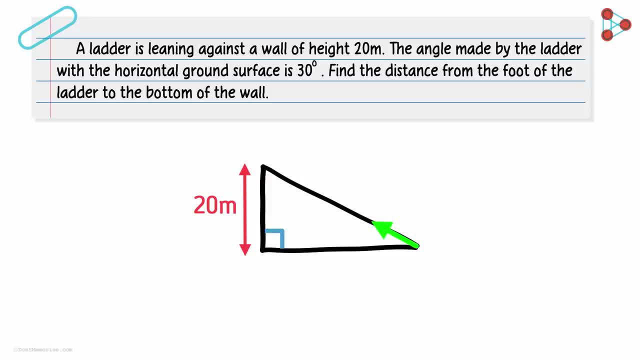 What else are we given? We are told that the angle made by the ladder with the surface is 30 degrees. That is, this angle is 30 degrees. And finally, we are asked to find this length, that is, the distance between the foot of ladder. 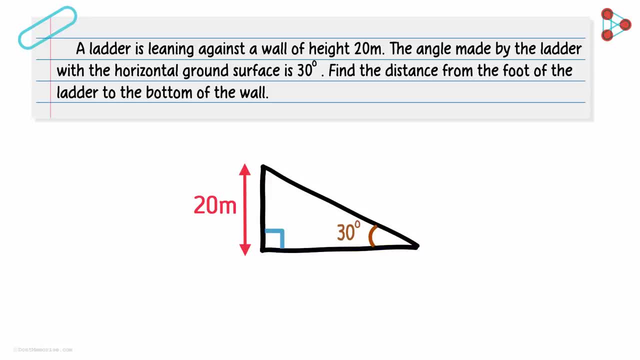 and the bottom of the wall. Now some of you may be wondering if we could have drawn the ladder on the other side like this: Guess what. It will not make any difference at all, So we will take the one we'd done originally. 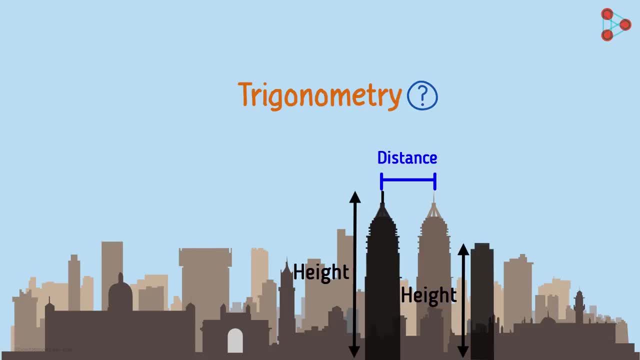 But first let's talk of one more important thing before I put a question. on the screen, We have seen trigonometric ratios of angles of a right angle triangle. Hence, forming the right triangle from the given question is the most important step while solving problems. 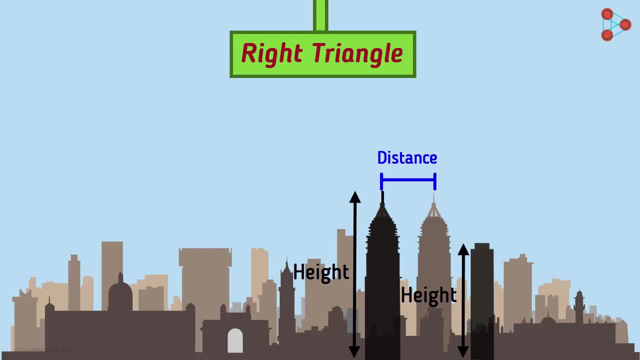 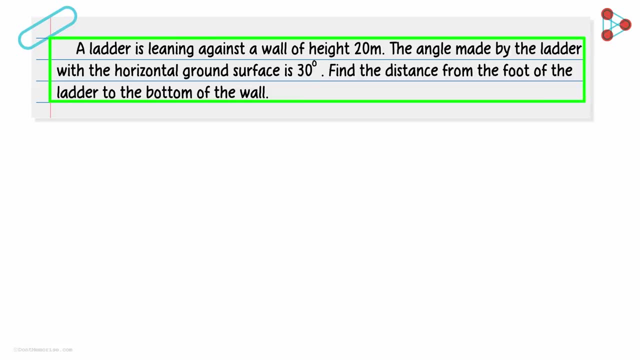 Now I will put a question on the screen And you try to sketch out a right triangle from the given information. Let's start with a simple example. Read the question carefully and try to form a right triangle. Here we are given a wall. 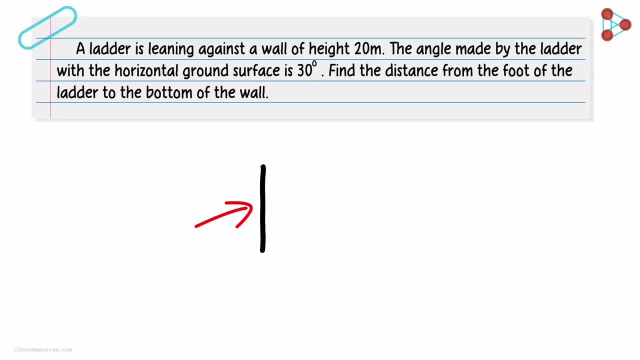 You can't represent the wall with a vertical line like we have done here? You don't really need to draw an actual wall Now. it's obvious that this wall makes an angle of 90 degrees with the ground surface. Let's try to draw a vertical line. 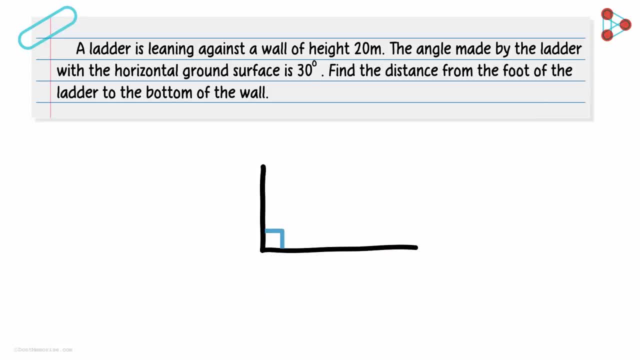 Here we are given an angle of 90 degrees with the ground surface. That's something we can definitely assume. We are also given the height of the wall, as 20 meters. A ladder is inclined against the wall like this. Again, you can represent the ladder with the inclined line, just like we have done here. 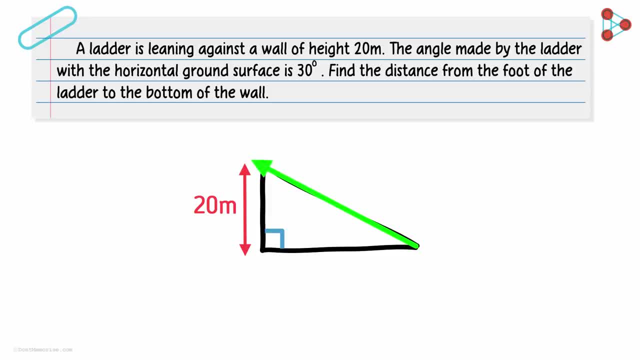 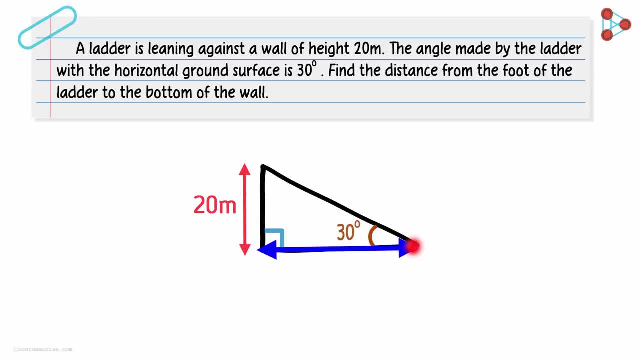 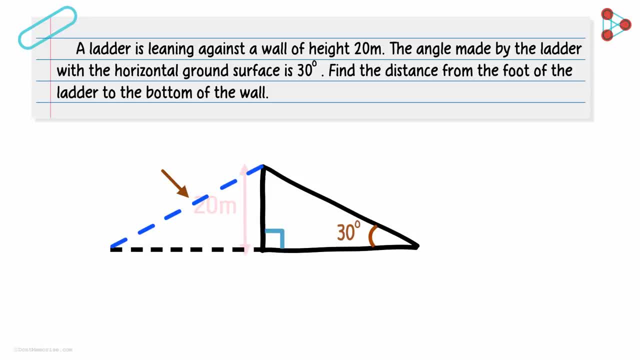 this Guess what. It will not make any difference at all, So we will take the one we had done originally. So here we have our right triangle, which pertains to this problem. It was easy to form, wasn't it? Let us name its vertices as A, B and C. 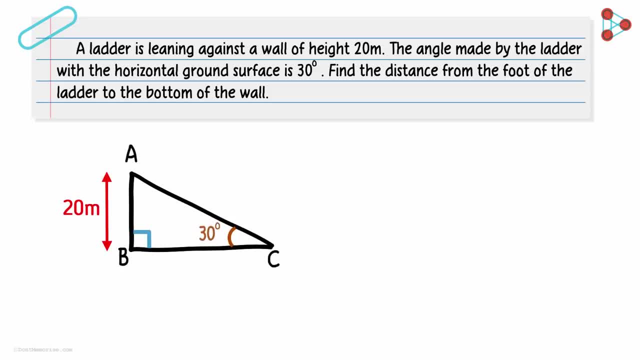 Ok, let us solve this quickly now. We are given the measure of angle C here, and we are also given the length of its opposite side, AB. We are asked to find length of BC. Which trigonometric ratios we will use here, Sine, cos or tan?